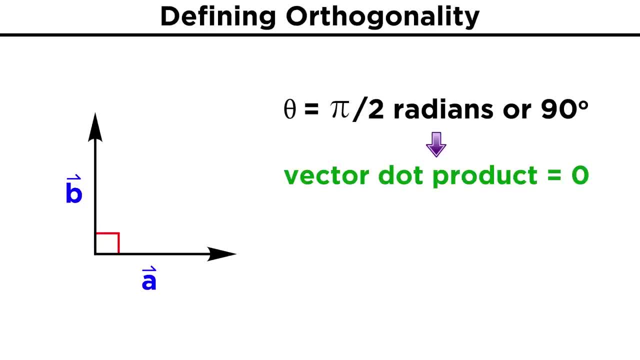 This situation will occur if the dot product between the two vectors is equal to zero, since the dot product is equal to the product of the two vector lengths times the quantity of the vector space. Let's now consider the vectors: A equals four, two negative one and B equals one negative. 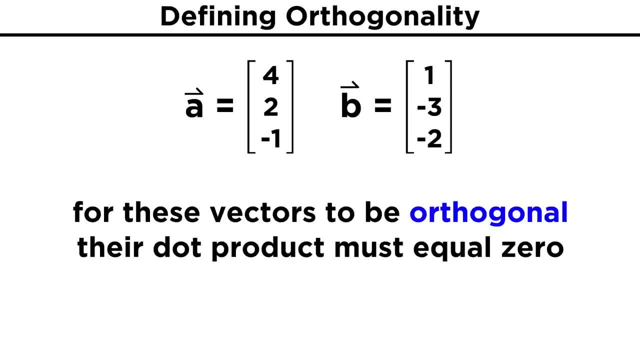 three negative two. To see if these vectors are orthogonal, we must check that the dot product is zero. To take the vector dot product, apart from the geometric definition we already mentioned, we can also use this algebraic one where we find the product of the first components. 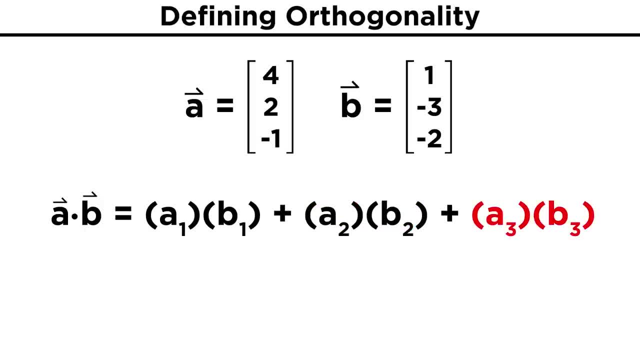 plus the product of the second components plus the product of the third components. In this particular case, this makes A dot B equal to four times one plus two times negative, three plus negative, one times negative two, which is four minus six plus two, or. 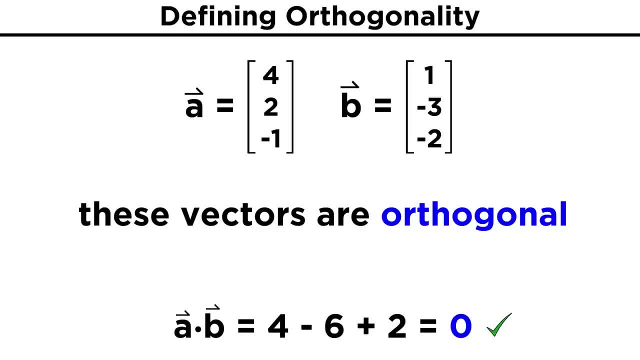 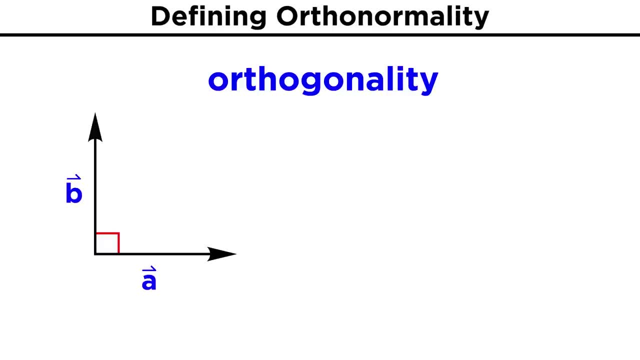 zero. Since the dot product is equal to zero. we can also use the algebraic equation to find our vectors are indeed orthogonal. Now let's expand on this basic concept. In addition to vectors being orthogonal, we can use another restriction on some vectors. 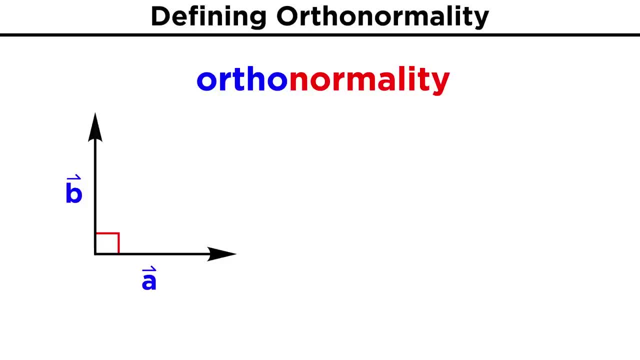 to create another useful concept: orthonormality. The normal part here refers to the vectors having a length of one. If a set of vectors are all of length one and also orthogonal, they are said to be orthonormal. We have already seen that one way to get the length of a vector is to take the square root. 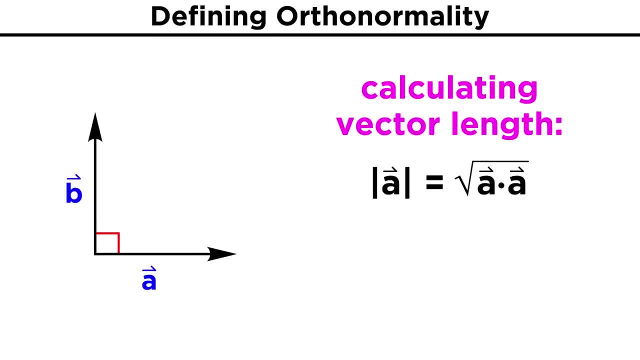 of the dot product involving the vector and itself, meaning the length of vector A is equal to the square root of A dot A. Now, if we then divide the original vector by that length, we will get a new vector that will be of length one. 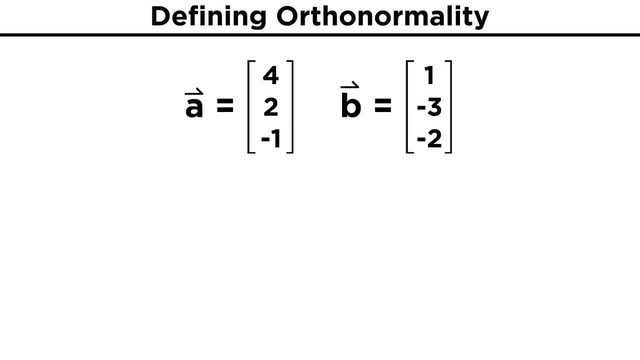 With that understood, let's take our two vectors from before, which were: A equals four, two negative one, and B equals one negative three negative two. The length of A will be given by the square root of four squared plus two squared plus 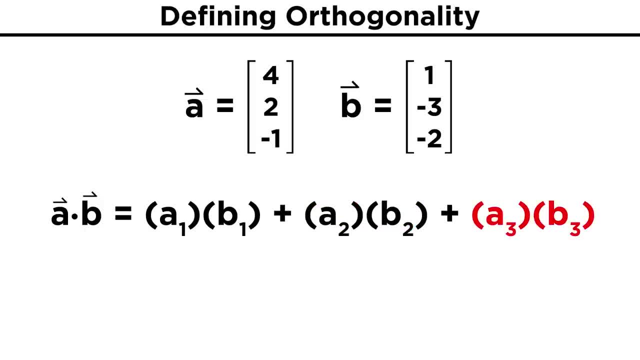 plus the product of the second components plus the product of the third components. In this particular case, this makes A dot B equal to four times one plus two times negative, three plus negative, one times negative two, which is four minus six plus two, or. 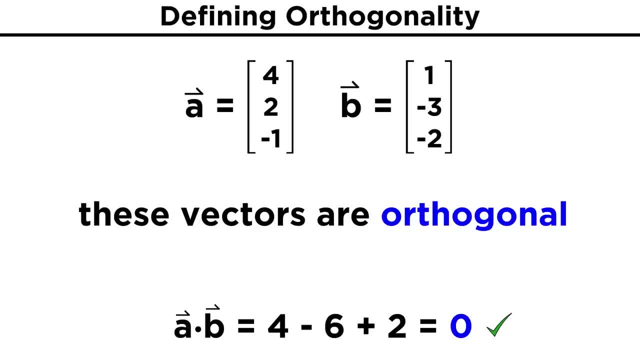 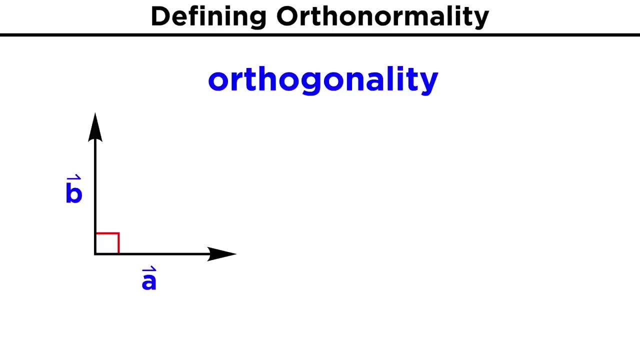 zero. Since the dot product is equal to zero, we can also use this algebraic one, and we can. vectors are indeed orthogonal. Now let's expand on this basic concept. In addition to vectors being orthogonal, we can use another restriction on some vectors to: 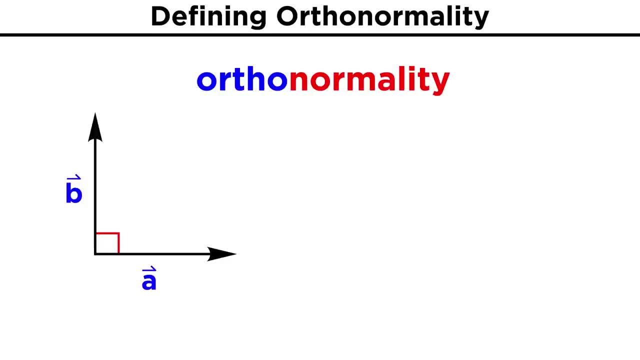 create another useful concept: orthonormality. The normal part here refers to the vectors having a length of one. If a set of vectors are all of length one and also orthogonal, they are said to be orthonormal. We have already seen that one way to get the length of a vector is to take the square root of the 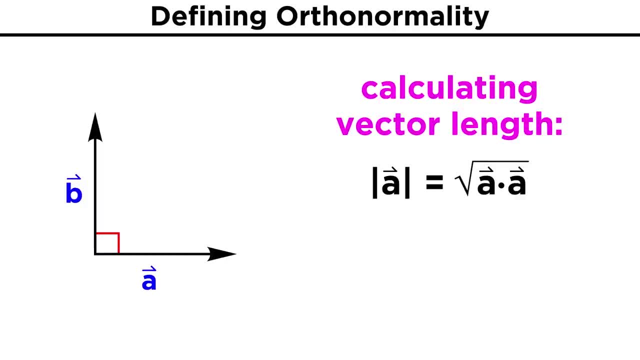 dot product involving the vector and itself, meaning the length of vector A is equal to the square root of A dot A. Now, if we then divide the original vector by that length, we will get a new vector that will be of length one. With that understood, let's take our two vectors from before, which were A equals. 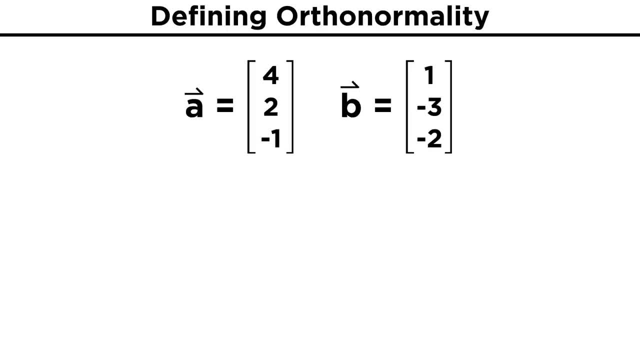 four, two negative one, and B equals one negative three negative two. The length of A will be given by the square root of four squared plus two squared plus negative one squared, which gives us the square root of sixteen plus four plus one, which is equal to root twenty-one. The length of B will be given by the square 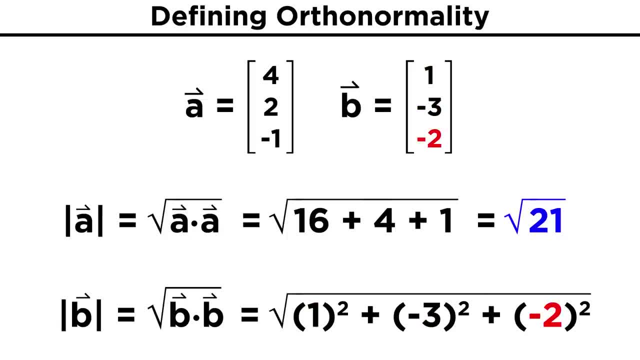 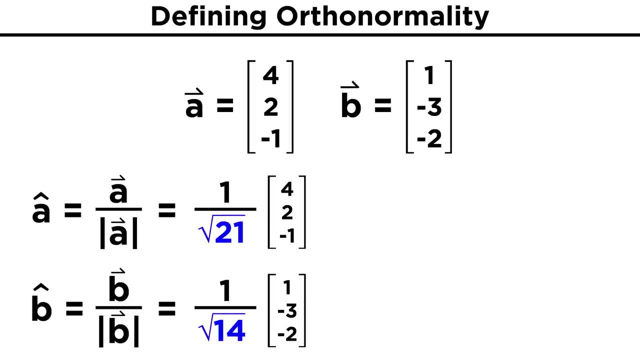 root of one squared plus negative three squared plus negative two squared, which gives us the square root of one plus nine plus four, which is equal to root fourteen. Now we can divide the vectors A and B by the lengths we just calculated and we get new. 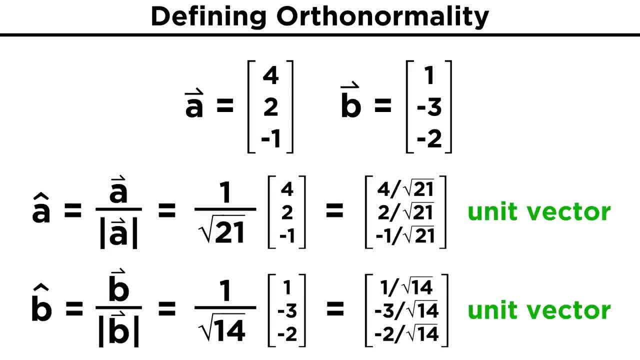 unit vectors four, two negative, one over root, twenty-one and one negative, three negative, two over root, fourteen. Here the word unit means that they have lengths that are equal to one. This process of making vectors into unit vectors is often called normalisation. By doing this, we have only 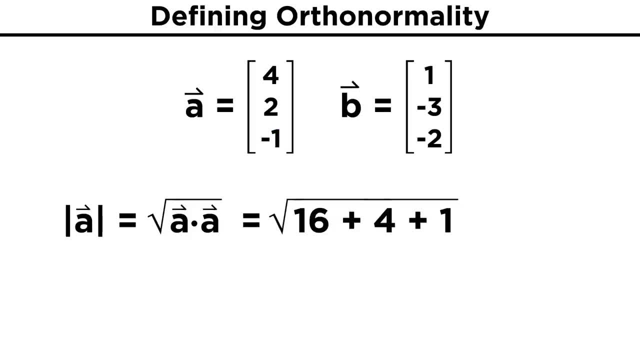 negative one squared, which gives us the square root of sixteen plus four plus one, which is equal to root twenty-one. The length of B will be given by the square root of one squared plus negative three squared plus negative two squared, which gives us the square root of one plus nine plus four, which is equal to root fourteen. 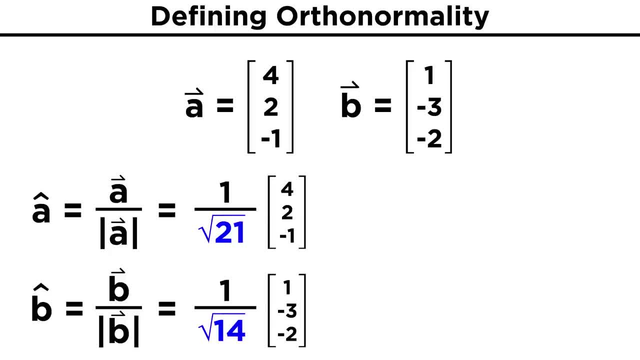 Now we can divide the vectors A and B by the lengths we just calculated and we get new unit vectors: four, two negative, one over root twenty-one and one negative, three negative, two over root fourteen. Here the word unit means that they have lengths that are equal to one. 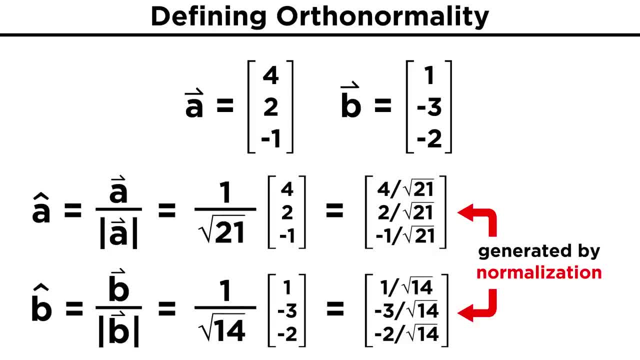 This process of making vectors into unit vectors is often called normalization. By doing this, we have only changed the magnitude of the vectors and not the direction. Because of this, they are still orthogonal, as we previously verified. And since these two vectors are orthogonal and also have lengths equal to one, that makes 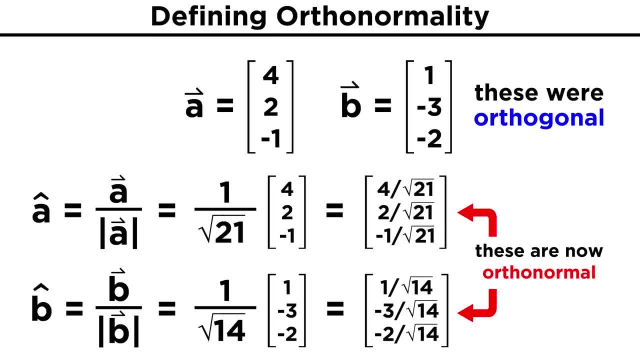 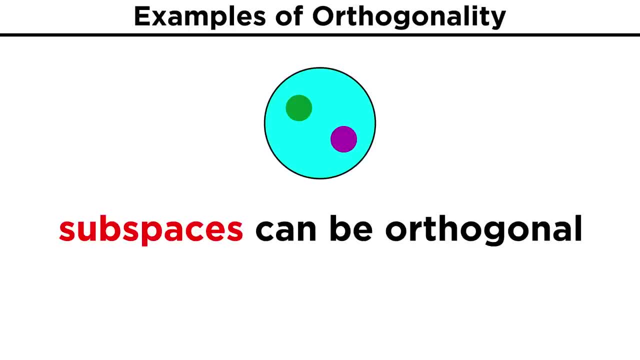 them orthonormal as well. It is actually not the case that only vectors can be considered orthogonal. We can also have orthogonal subspaces. Two subspaces, A and B, are said to be orthogonal. if every vector in A is orthogonal to every. 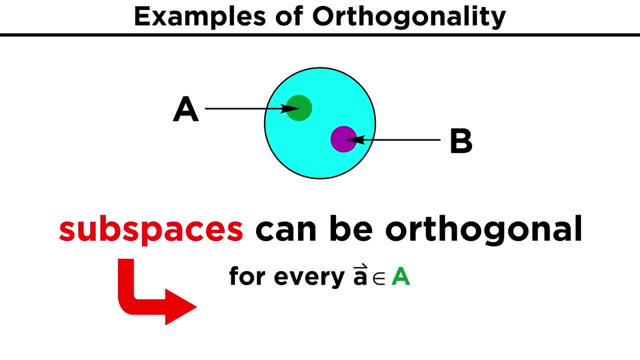 vector in B. So for any vector A in subspace A and any vector B in subspace B, A dot B must be equal to zero. Consider the following subspaces of R3.. Subspace A is made of the vectors of the form which can have any value as the 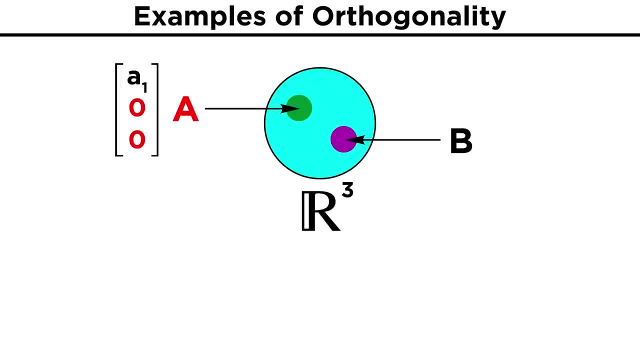 first component, but must have zeros as the second and third. Subspace B is made of the vectors of the form which have a zero as the first component and can have any value as the second and third. While there are an infinite number of vectors that can satisfy these conditions, they are: 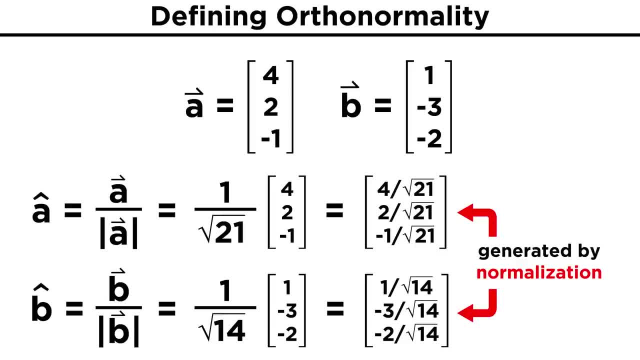 changed the magnitude of the vectors and not the direction. Because of this, they are still orthogonal, as we previously verified, And since these two vectors are orthogonal and also have lengths equal to one, that makes them equal to one, Save the hopefully- puns. 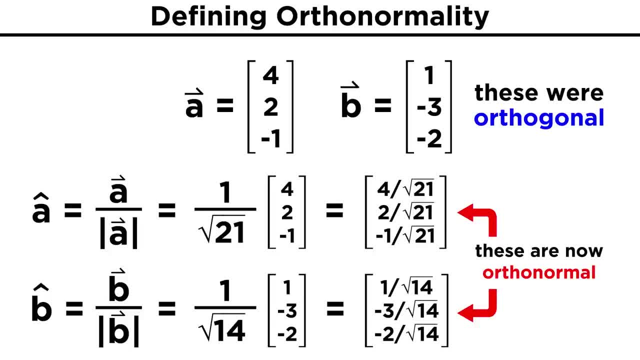 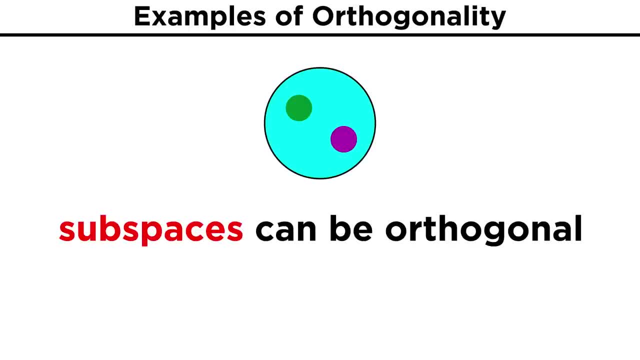 orthonormal as well. It is actually not the case that only vectors can be considered orthogonal. We can also have orthogonal subspaces. Two subspaces, A and B, are said to be orthogonal if every vector in A is orthogonal to every vector in B. So for any vector A in subspace A and any vector B in subspace B, A dot B. 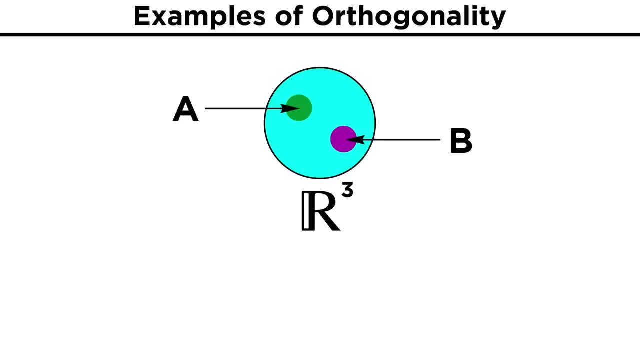 must be equal to zero. Consider the following subspaces of R3.. Subspace A is made of the vectors of the form which can have any value as the first component, but must have zeros as the second and third. Subspace B is made of the vectors of the form which have a zero as the first component. 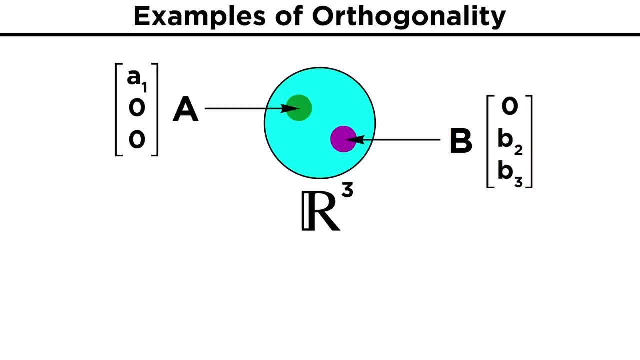 and can have any value as the second and third, While there are an infinite number of vectors that can satisfy these conditions, there are subspaces. Taking the dot product of any possible vector in subspace A and any possible vector in subspace B gives us A1 times zero plus zero times B2, plus zero times B3, and this will 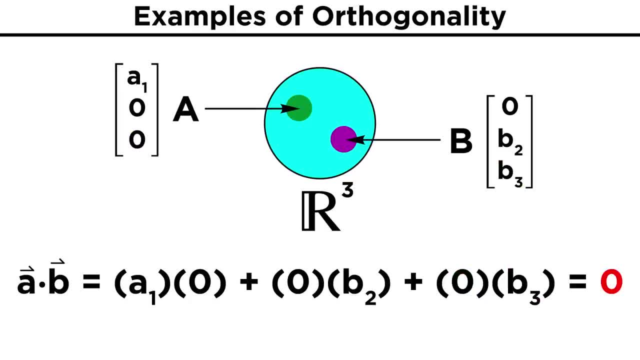 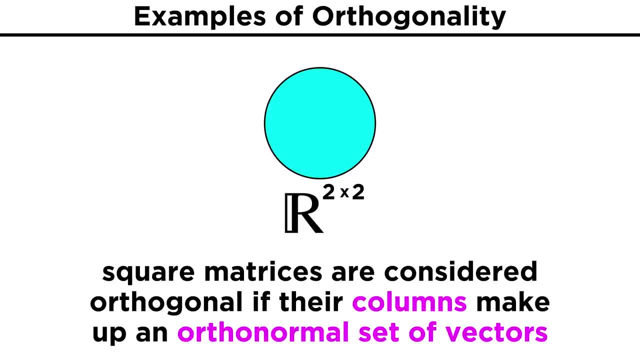 be equal to zero, no matter what those values are. Because of this, we have shown that the subspaces A and B are orthogonal. Square matrices can also be orthogonal. The condition for this is simply that the columns of the matrix make up an orthonormal. 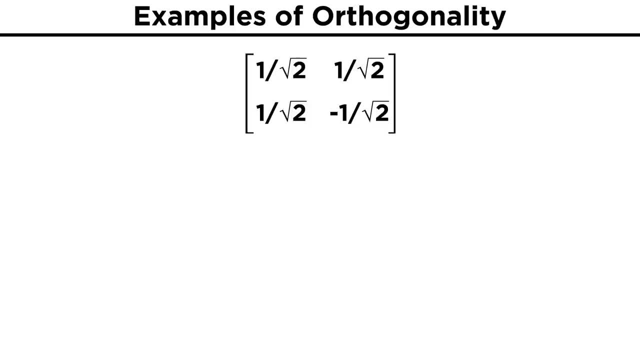 set. Take, for example, the two by two matrix made up of one over root, two in all elements, but the bottom right is negative. Taking the columns of this matrix as vectors, one over root two, one over root two and one over root two negative, one over root two- let's verify that they are orthonormal. 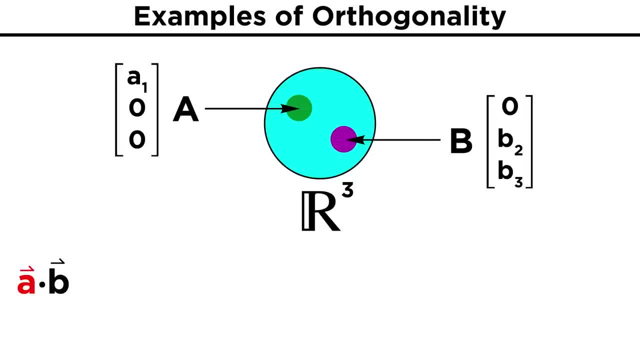 not orthogonal. Taking the dot product of any possible vector in subspace A and any possible vector in subspace B gives us A1 times zero plus zero times B2, plus zero times B3, and this will be equal to zero, no matter what those values are. 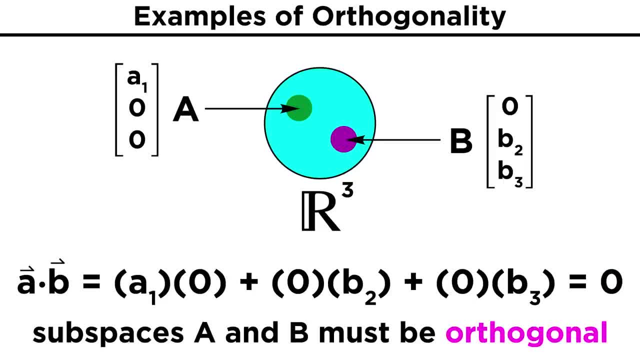 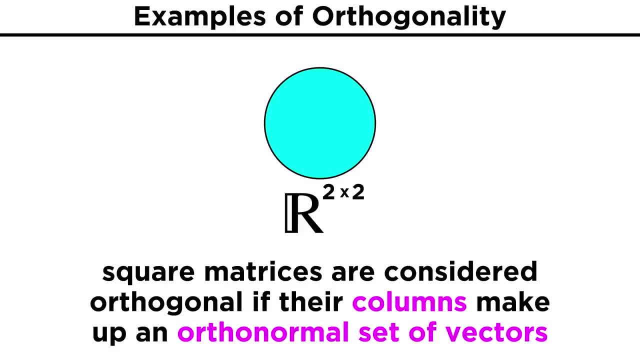 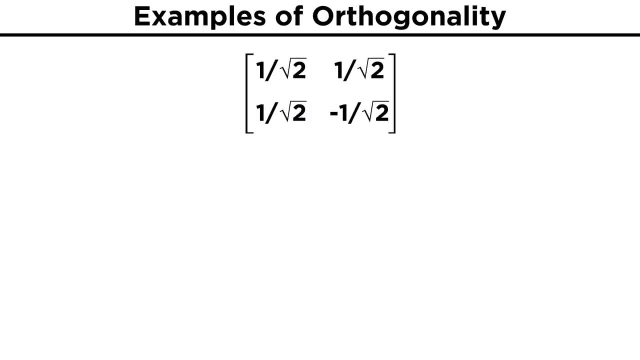 Because of this, we have shown that the subspaces A and B are orthogonal. Square matrices can also be orthogonal. The condition for this is simply that the columns of the matrix make up an orthonormal set. Take, for example, the 2x2 matrix made up of in all elements but the bottom. 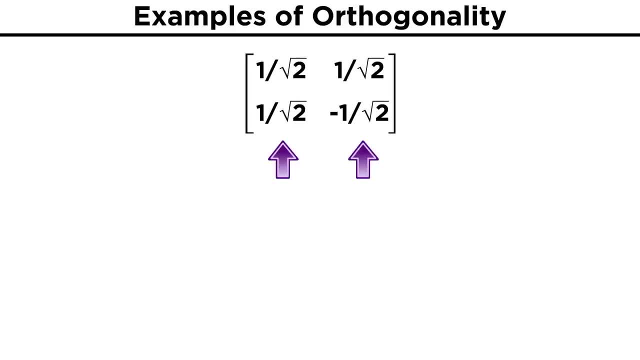 right is negative. Taking the columns of this matrix as vectors: 1 over root 2,, 1 over root 2, and 1 over root 2, negative: 1 over root 2, let's verify that they are orthogonal. 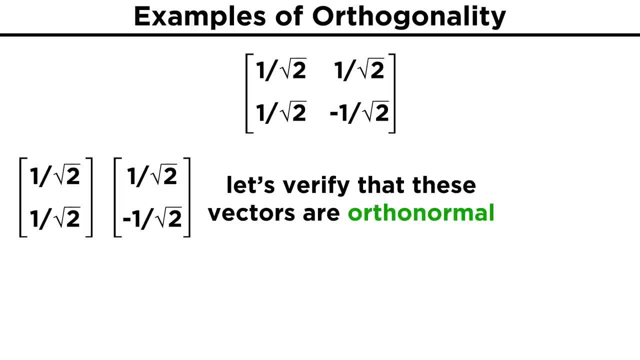 This might look deceptive. Well, that will do. First, to check for orthogonality, we can take the dot product, which will give us one over root, two times one over root, two plus one over root, two times negative, one over. 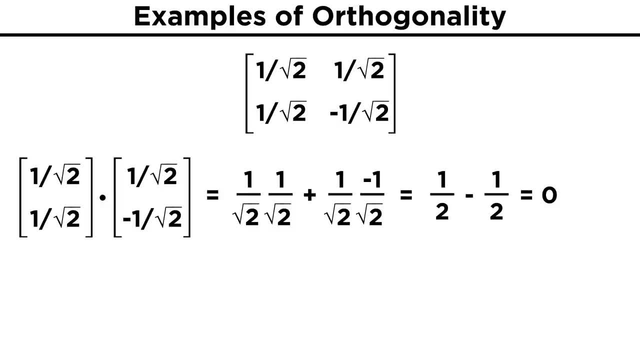 root two. This becomes one half minus one half, which is simply zero, meaning that these vectors are orthogonal. Now we just need to verify that they both have lengths of one. The length of the first will be the square root of one over root two. quantity squared. 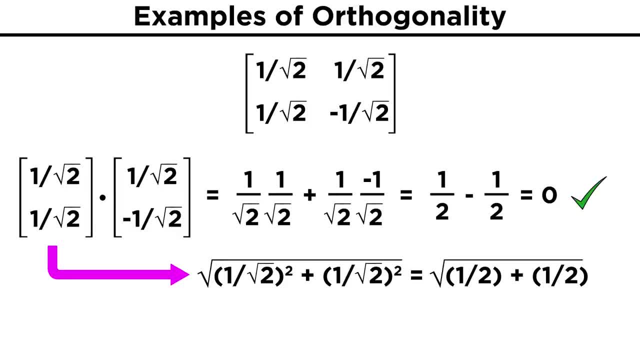 plus one over root two quantity squared, which is the square root of one half plus one half, or the square root of one, which is one. Then, for the second, the length is the square root of one over root two quantity squared, plus negative one over root two quantity squared, which again becomes the square root of one. 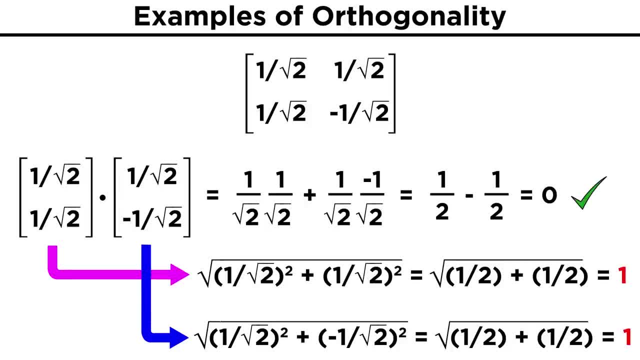 half plus one half, or the square root of one, which is one. Both vectors have a length of one and are orthogonal to each other. This makes the columns of the matrix an orthonormal set, meaning that the matrix itself is orthogonal. 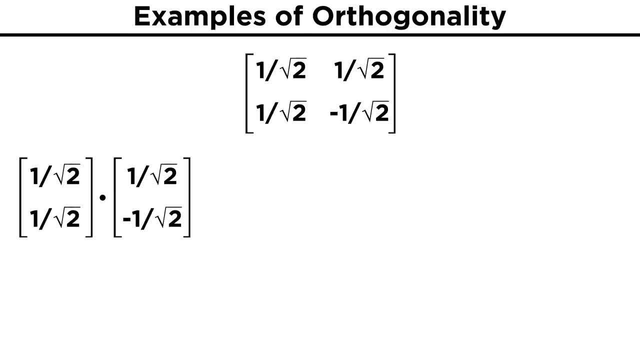 First, to check for orthogonality, we can take the dot product, which will give us one over root two times one over root two plus one over root, two times negative one over root two. This becomes one half minus one half, which is simply zero, meaning that these vectors 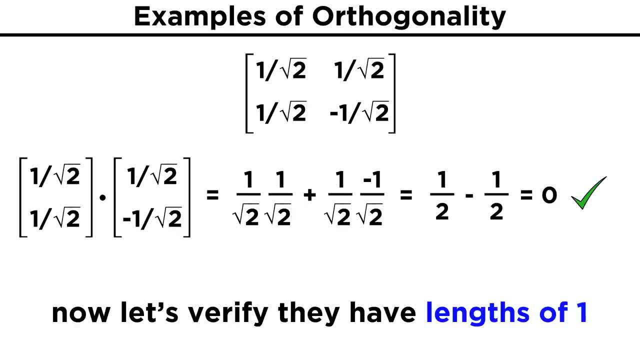 are orthogonal. Now we just need to verify that they both have lengths of one. The length of the first will be the square root of one over root, two quantity squared, plus one over root, two quantity squared, which is the square root of one half plus one half. 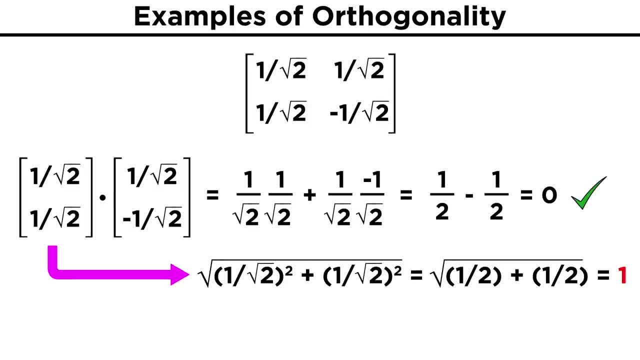 or the square root of one which is one. Then for the second, the length is the square root of one over root- two quantity squared plus negative, one over root, two quantity squared, which again becomes the square root of one half plus one half, or the square root of one which is one. 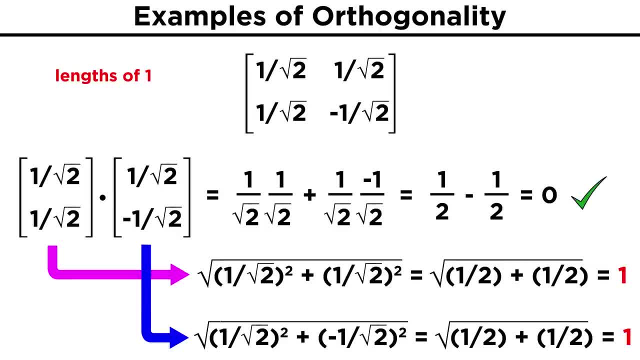 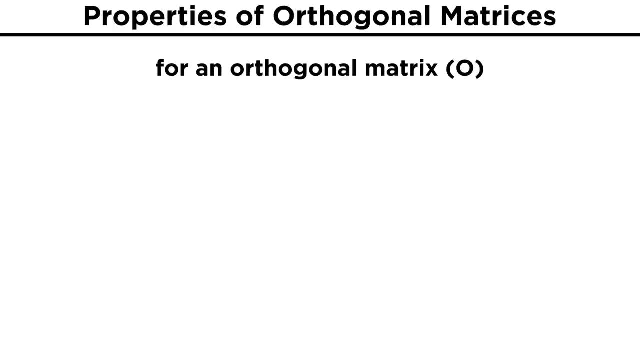 Both vectors have a length of one and are orthogonal to each other. This makes the columns of the matrix an orthonormal set, meaning that the matrix itself is orthogonal. The main benefit to having an orthogonal matrix is that the inverse of the matrix is simply. 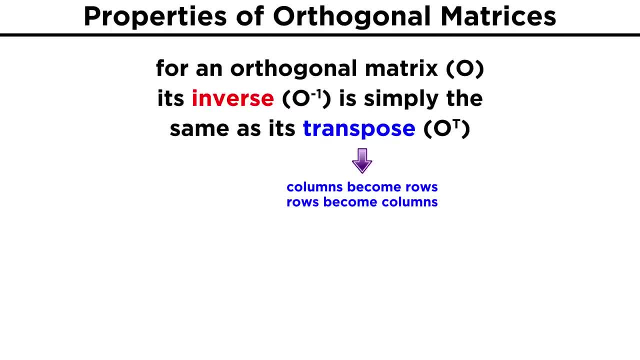 the same as its transpose. By transpose we mean that the columns of the matrix become the rows and vice versa. For example, the transpose of a two-by-two matrix and a three-by-three matrix are given as shown. You can see that the first row becomes the first column, the second row becomes the second. 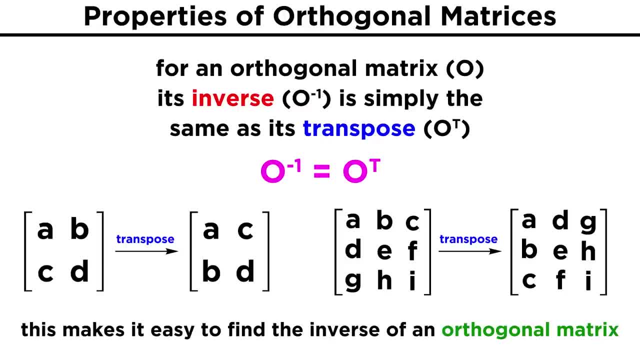 column and so on. For an orthogonal matrix, generating the inverse is as simple as finding the transpose, and this makes it extremely easy to find the transpose. You can also find the inverse of orthogonal matrices as you simply swap some elements around. 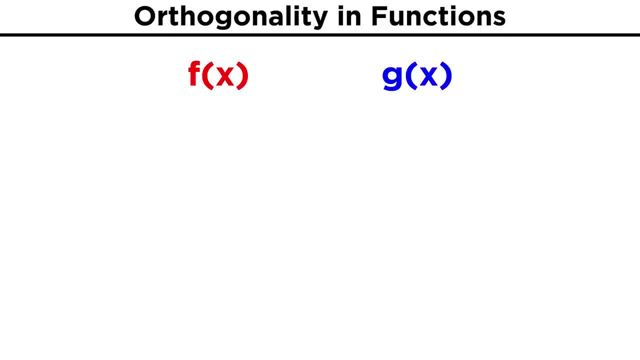 Lastly, we can even consider orthogonality between functions. However, to do this, we must consider a definition for something called the inner product. from point A to point B, for the functions f of X and g of X, This inner product, written as between angular brackets, is defined to be the integral. 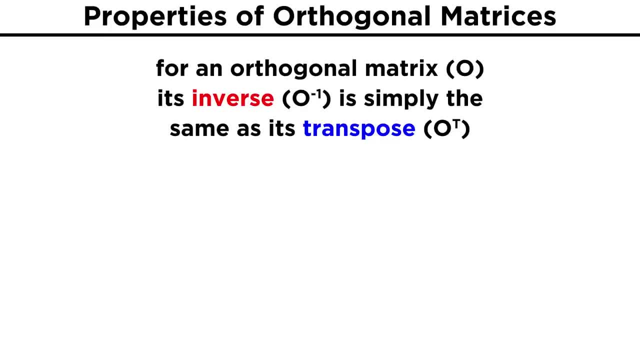 The main benefit to having an orthogonal matrix is that the inverse of the matrix is simply the same as its transpose. By transpose we mean that the columns of the matrix become the row, So the matrix is orthogonal to each other. For example, the transpose of a two by two matrix and a three by three matrix are given. 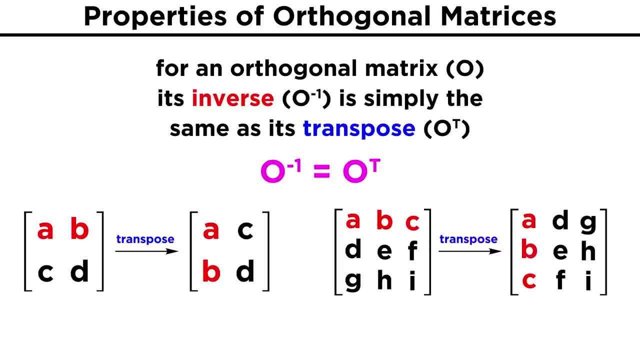 as shown. You can see that the first row becomes the first column, the second row becomes the second column, and so on. For an orthogonal matrix, generating the inverse is as simple as finding the transpose, And this makes it extremely easy to find the inverse of orthogonal matrices, as you simply. 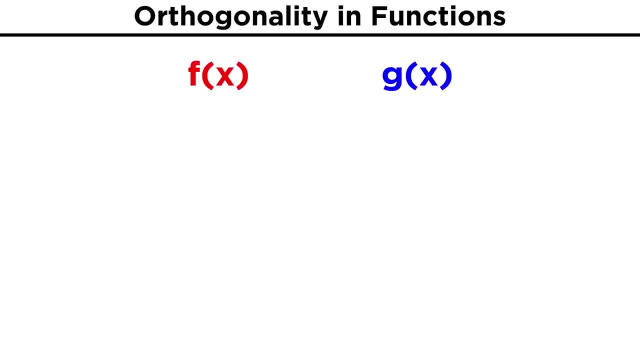 swap some elements around. Lastly, we can even consider orthogonality between functions. However, to do this, we must consider a definition for something called the inner product. from point A to point B for the functions f and g, This inner product, written as between angular brackets, is defined to be the integral. 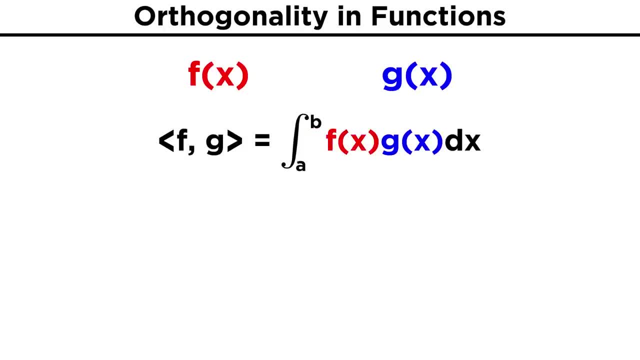 from A to B of Okay, Okay. Once again, if this inner product ends up being equal to zero, the functions are said to be orthogonal. However, in this case, there is some dependence on what range of values we are considering. 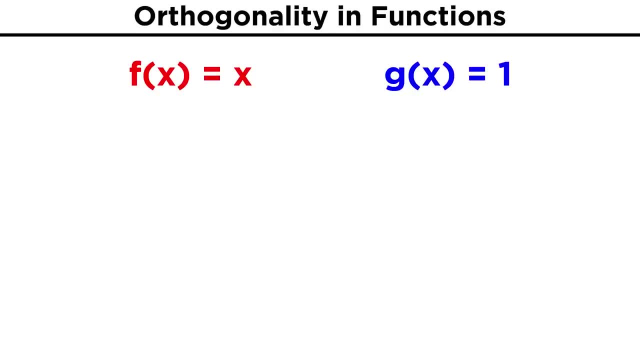 Take, for example, the functions f of x equals x and g of x equals one. Our inner product, fg will be equal to the integral from a to b of xdx. As we recall from our study of calculus, the antiderivative here will be x squared over. 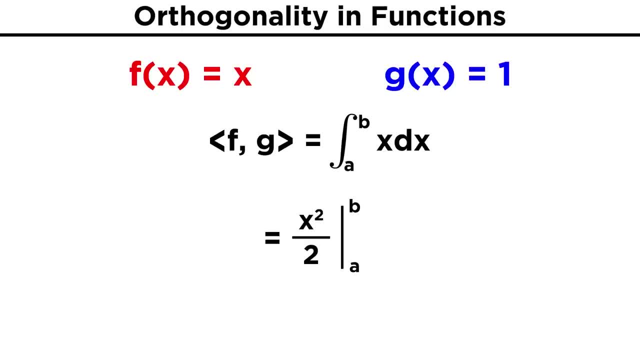 two and we must evaluate this at b and then subtract from that the evaluation at a. Let's say our interval goes from a equals negative one to b equals one. Then our inner product becomes one squared over two, minus negative one squared over two. 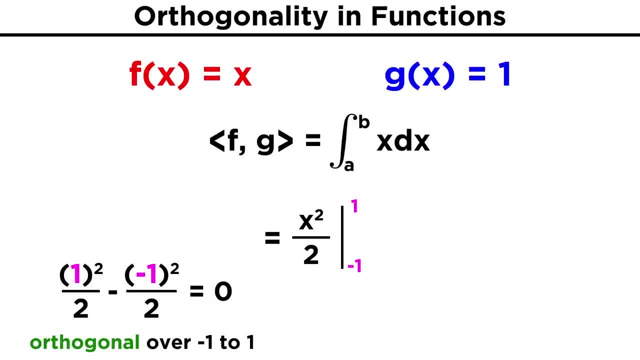 which is equal to zero. so our functions are orthogonal across this range. However, if we consider the range from a equals zero to b equals one, then our inner product is now one squared over two minus zero squared over two, which is equal to one. 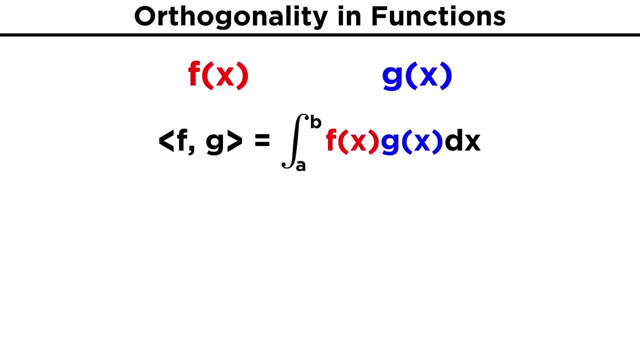 a to b, of f, of x times g, of x, dx. Once again, if this inner product ends up being equal to zero, the functions are said to be orthogonal. However, in this case there is some dependence on what range of values we are considering. 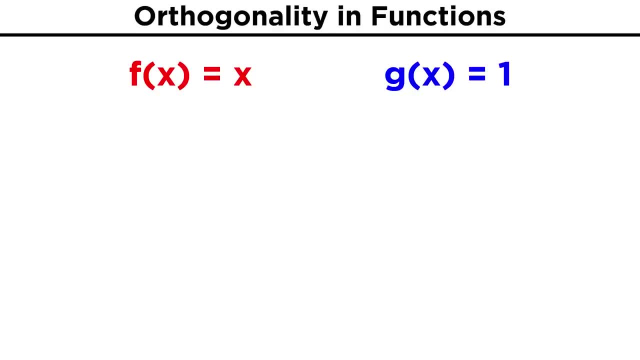 Take, for example, the functions f of x equals x and g of x equals one. Our inner product, f, g will be equal to the integral from a to b of x- dx. As we recall from our study of calculus, the antiderivative here will be x squared over. 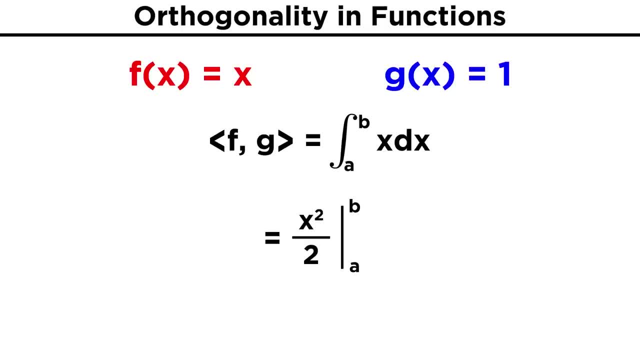 two and we must evaluate this at b and then subtract from that the evaluation at a. Let's say our interval goes from a equals negative one to b equals one. Then our inner product becomes one squared over two, minus negative one squared over two. 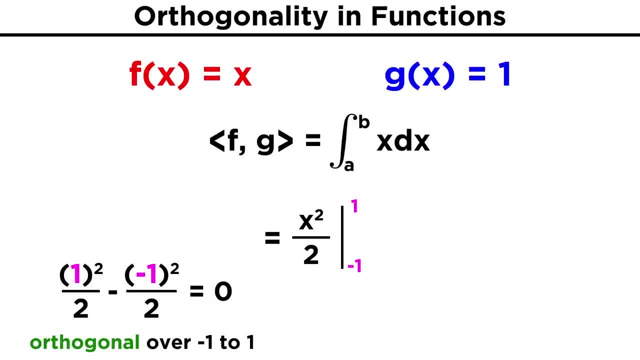 which is equal to zero. so our functions are orthogonal across this range. However, if we consider the range from a equals zero to b equals one, then our inner product is now one squared over two minus zero squared over two, which is equal to one. 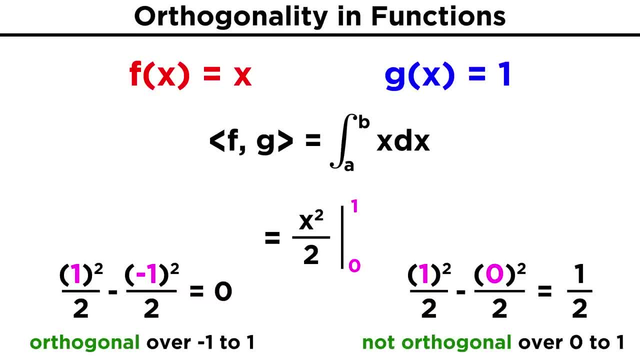 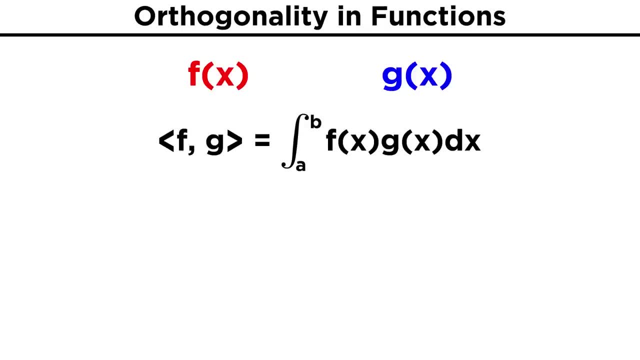 half and therefore no longer zero, So our functions are not orthogonal over this range of values. There are many things to consider when looking at the inner product of two functions. In fact, oftentimes an extra function, w of x, referred to as the weight function, is. 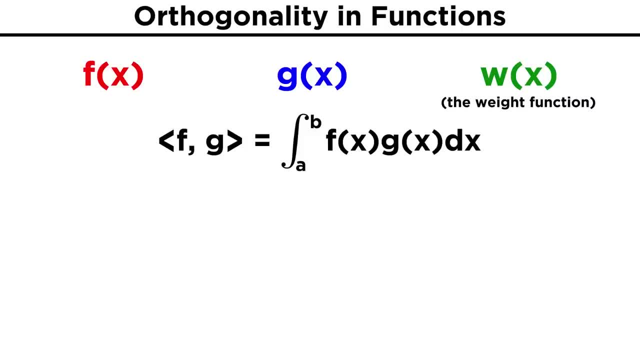 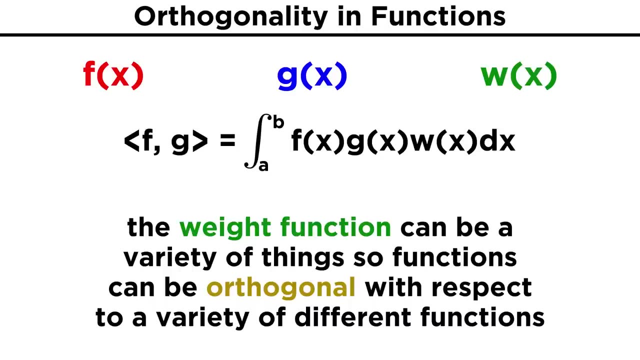 not orthogonal. The weight function is added to the definition of the inner product so that f comma g equals the integral from a to b of f, of x times g, of x times w, of x dx. This weight function can be any of a variety of different things, meaning we can have functions. 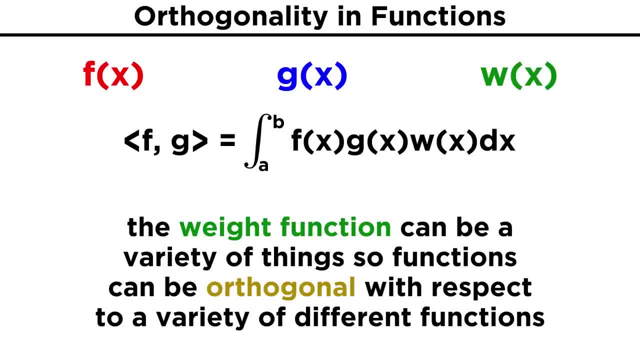 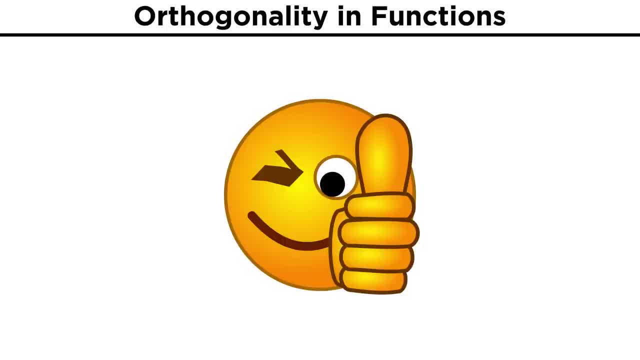 that are orthogonal with respect to a variety of different functions. Orthogonality ends up playing a key role in several aspects of math and even science. It helps us break down systems into distinct elements for easier understanding and problem solving. So to make sure we understand, let's check comprehension.